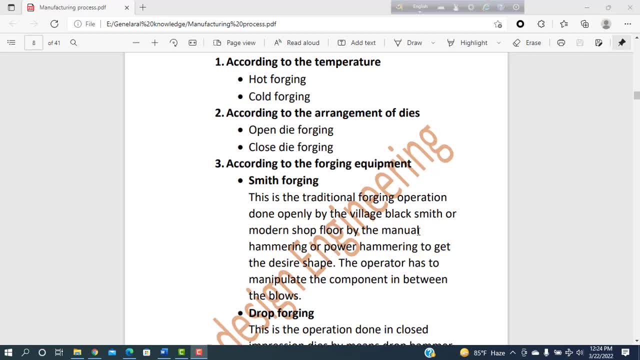 the arrangement of the dies. it is two types: open die forging and closed die forging, According to the forging equipment. this one is the smith forging and I am describing shortly This is the traditional forging operation. I mean smith forging is the traditional operation, So this is done openly by the billets, black smith or modern shoppers and also these are 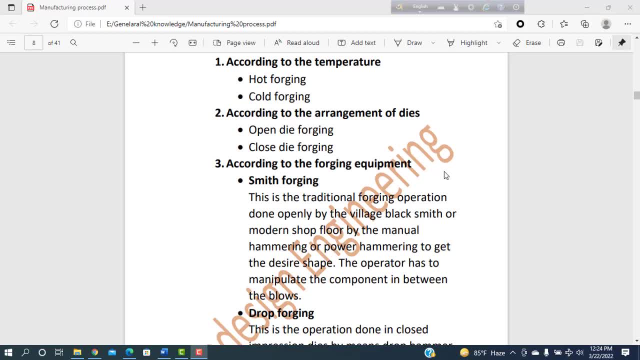 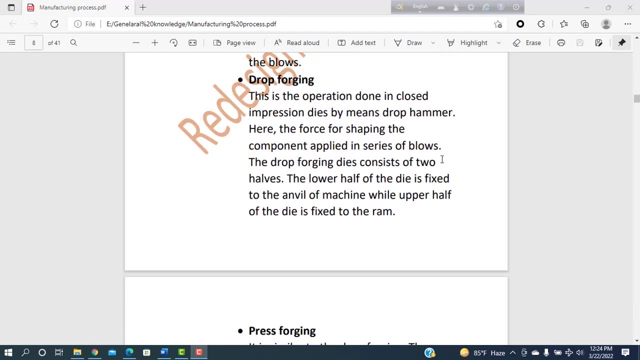 the other options. The other option is the lucky ring choice, which is used to make the floor by the manual hammering or power hammering. to get the desired shape, The operator has to manipulate the component in between the blows: Drop Forging. This is the operation done in closed impression. 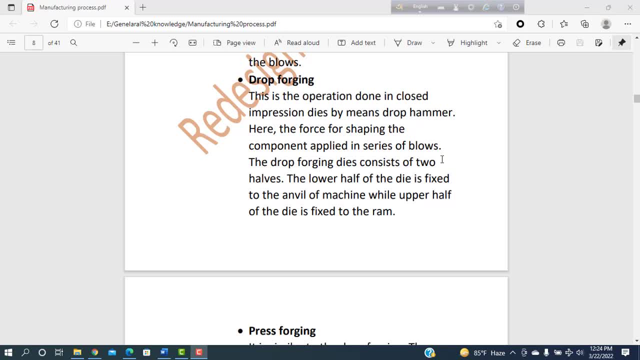 die by means drop hammer. We are the force for shaping the component applied in series of blows. The drop forcing die consists of two halves. the lower half of the die is fixed to the anvil of the machine, while upper half of the die is fixed to the ram. 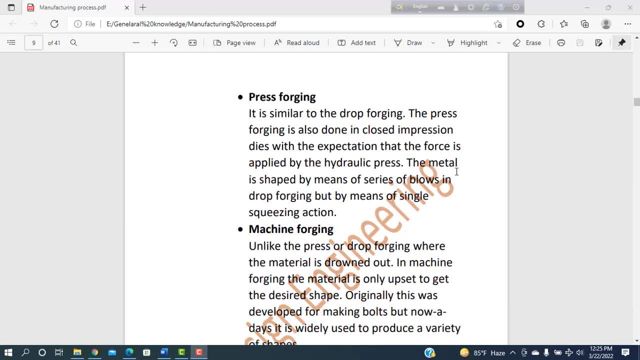 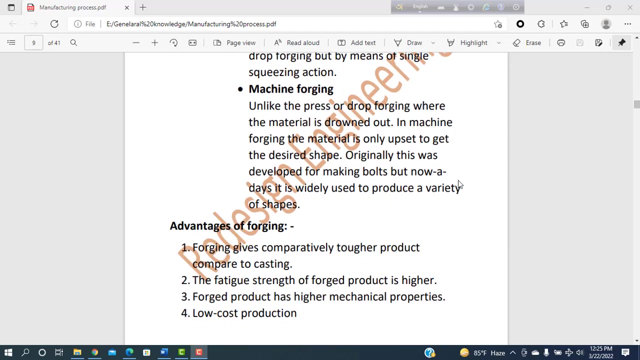 Press Forging. It is similar to the drop forcing. The press forcing is also done in closed impression dies, with the expectation that the force is applied by means by the hydraulic press. The metal is shaped by means of series of blows in drop forcing, but by means of single squeezing action. 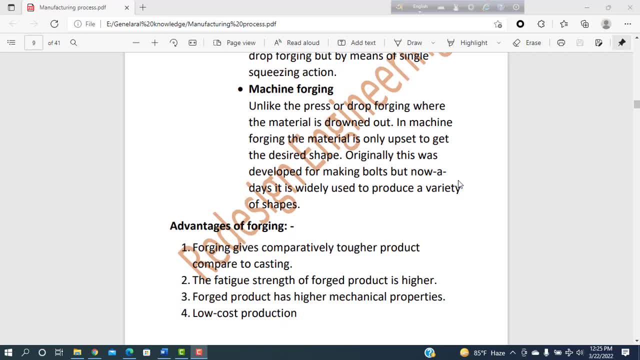 Machine Forging, Unlike the press or drop forcing further, the material is drawn out. In machine forcing the material is only upset to get the desired shape. Originally this was developed for making bolts, but nowadays it is widely used to produce a variety of shapes. Generally, originally, 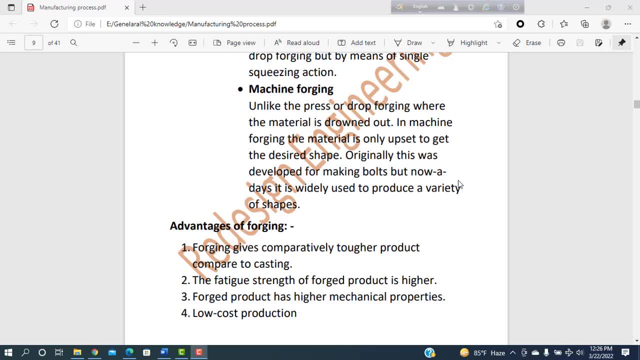 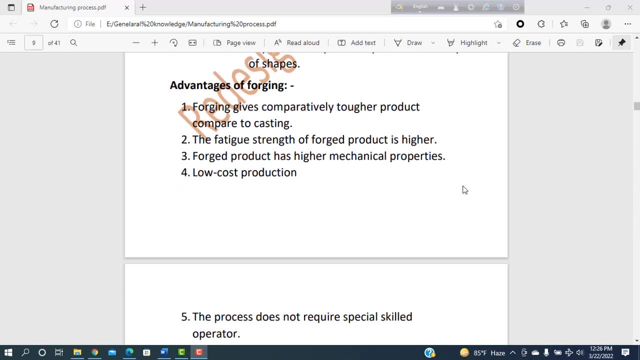 it was developed for making bolts, but now it is producing a variety of shapes of products. Advantages of Forging: Forging gives- I mean provides- comparatively tougher products compared to casting. The fatigue strength of the material is very low. The strength of a forced product is higher. Forged product has higher mechanical properties. 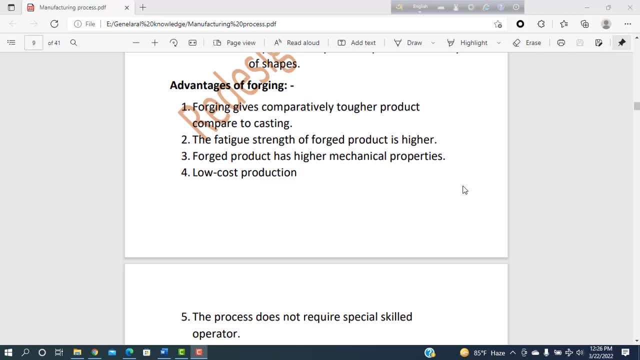 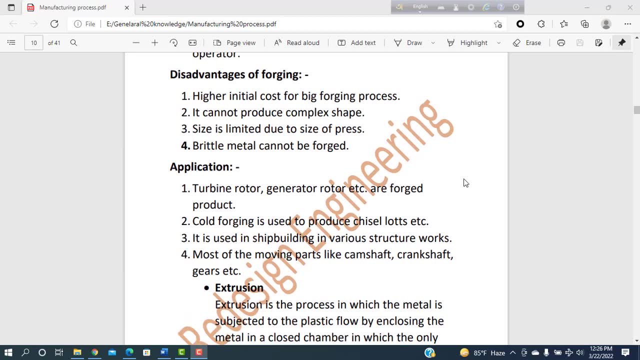 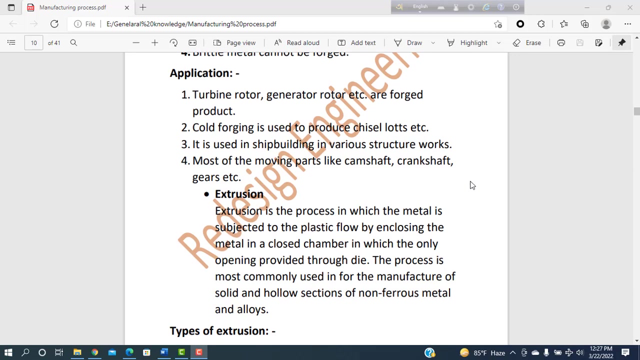 low cost production. The process does not require special skilled operator. Disadvantages of Forging: Higher initial cost for big forging process. It cannot produce complex shapes. Size is limited due to size of press. Brittle material cannot be forged. Application Turbine rotor, generator rotor, etc are forced products. Cold forging is used to produce. 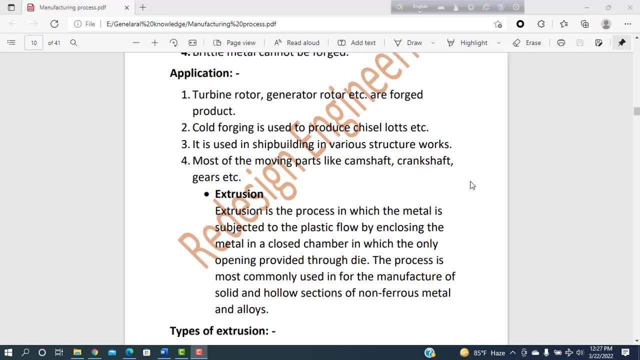 scissor lots, etc. It is used in ship building. in various structure works Most of the moving parts like camshaft, crankshaft, gear, etc. Extrusion. Extrusion is the process in which the metal is subjected to the plastic flow by enclosing the metal in a closed chamber in which the 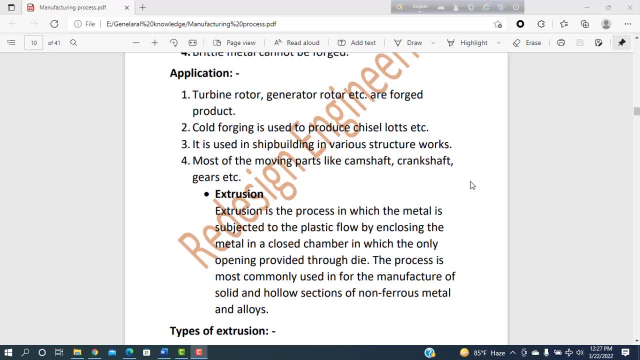 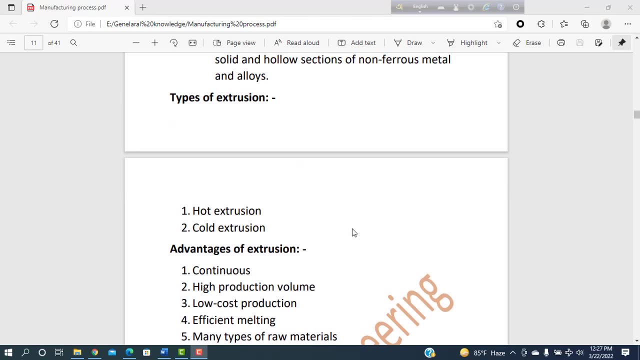 only opening provided through die. The process is most commonly used in for the manufacture of solid and hollow sections of non-ferrous metal or alloy Types of Extrusion Extrusion is generally proposed. The first is hot extrusion, second is the cold extrusion. 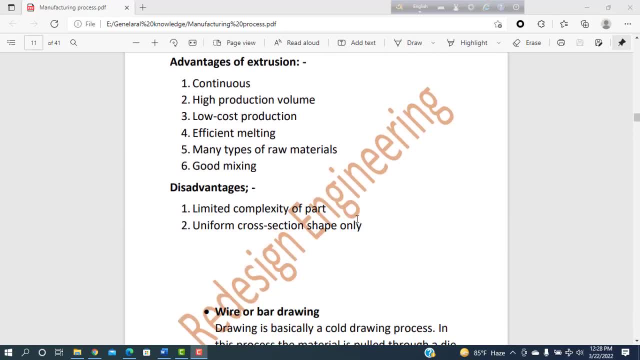 Advantages of Extrusion: It is the continuous process. high production volume, low cost production, efficient melting, many types of raw materials and gold mixing. Disadvantages: Limited complexity of parts. uniform cross section shape, only Wire or Bar Drawing. Drawing is basically a cold extrusion. It can be used for any type of construction. 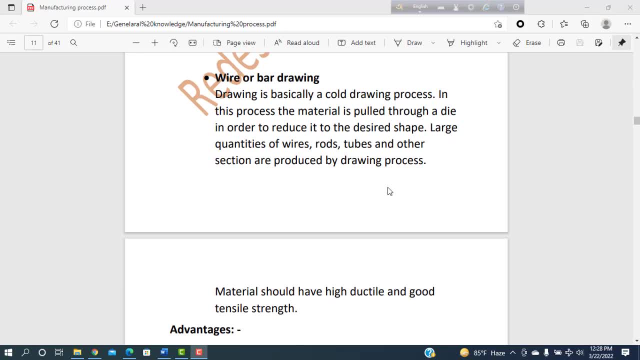 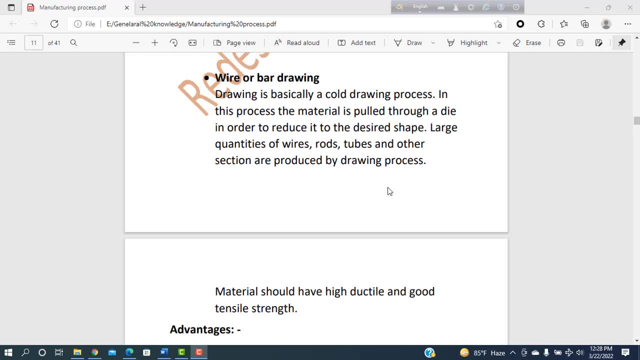 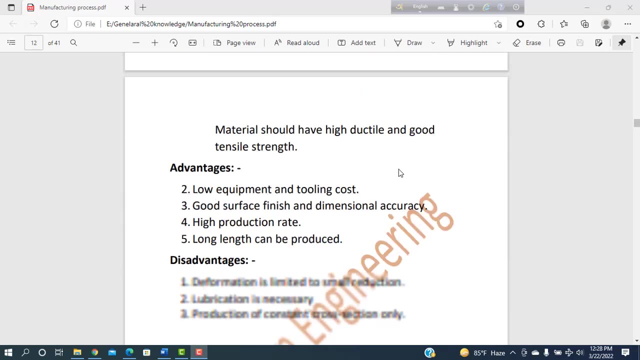 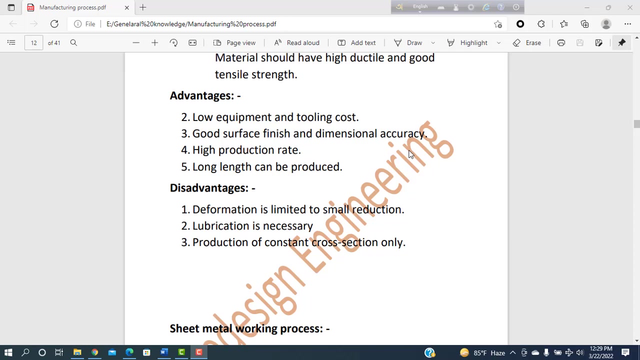 of wires, rods, tubes and other sections are produced by drawing process. Material should have high ductile and gold can cell strength. I mean this condition is required for the wire or bar. drawing Advantages: Low requirement and pulling cost. good surface finish and dimensional accuracy. high production. 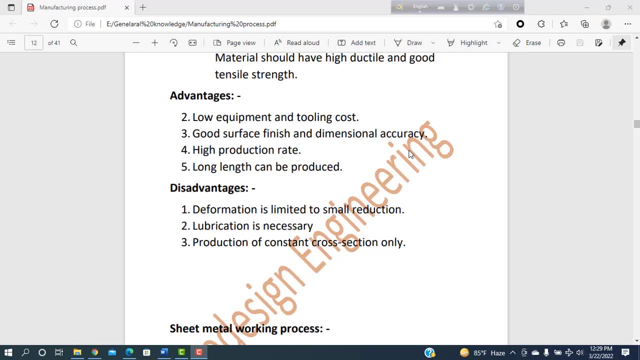 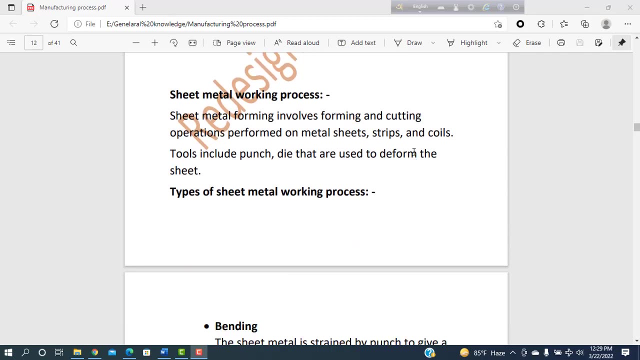 rate. long length can be produced. Here also the some disadvantages: deformation is limited to a small reduction. lubrication is necessary. production of constant cross section only Sheet metal working process. Sheet metal forming involves forming and cutting operations performed on metal sheets strips. 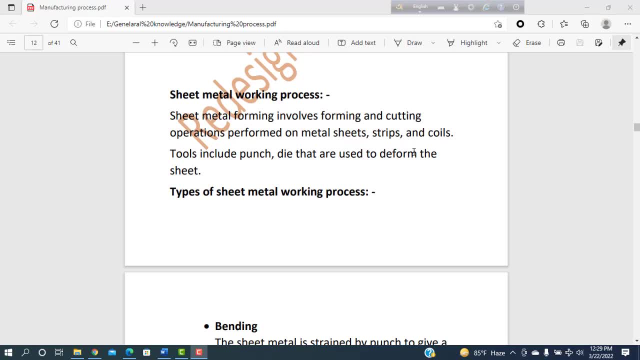 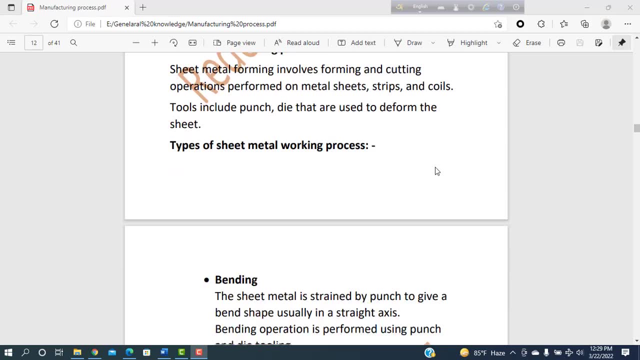 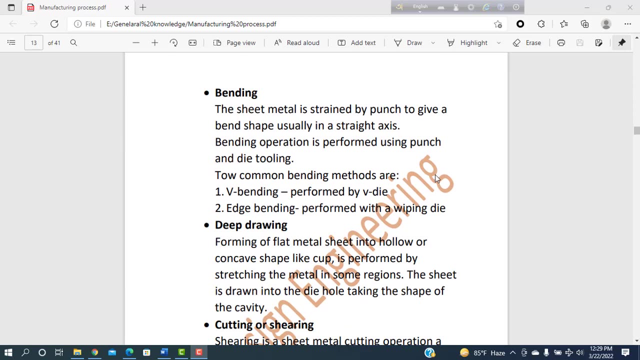 and coils. Tools include pans, die that are used to deform the sheets. Type of sheet metal working process. And sheet metal working process includes that bending the sheet metal is strained by pans to give a bent shape, usually in a straight axis. Bending operation is performed using pans and die tooling. 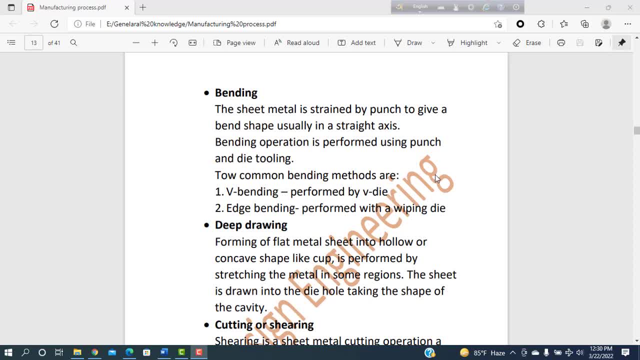 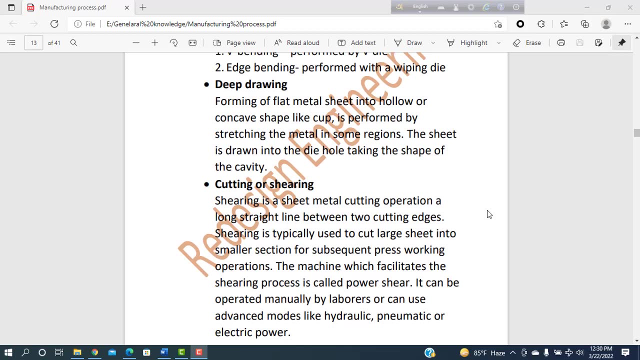 Two common bending methods are used: V bending and S bending. V bending is performed by the V die and S bending is performed with a weeping die. Deep drawing Forming of flat metal sheet into hollow or concave shape like curve is performed by scratching the metal. in some regions 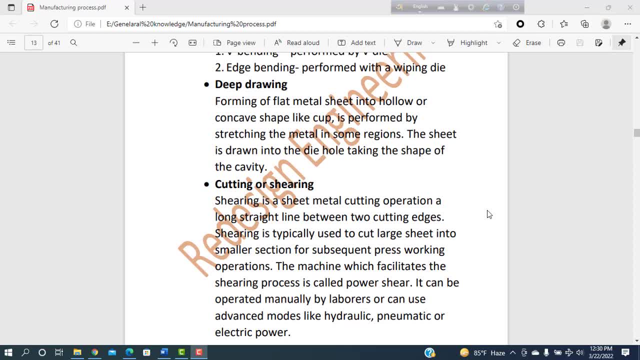 The sheet is drawn into the die hole, Taking the shape of the cavity. Cutting or Shearing. Shearing is the sheet metal cutting operation along a straight line between two cutting edges. Shearing is typically used to cut large sheets into smaller sections for subsequent press. 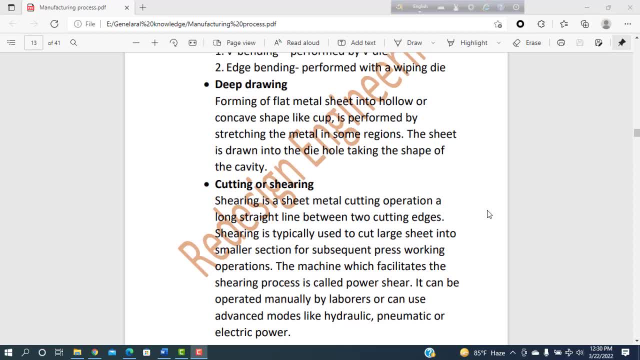 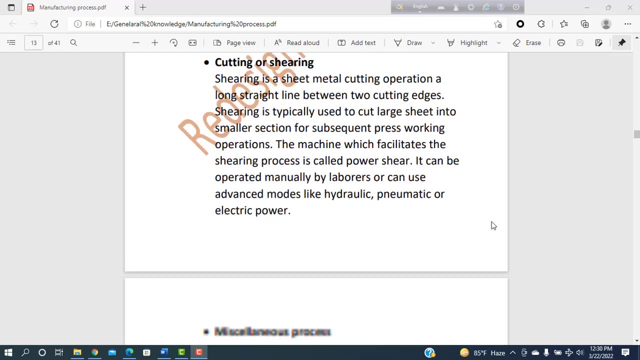 working operations. The machine. who is facilities? the shearing process is called power shear. It can be operated manually by laborers or can be used at budget. It can be used in advanced modes like hydraulic, pneumatic or electric power. miscellaneous process. 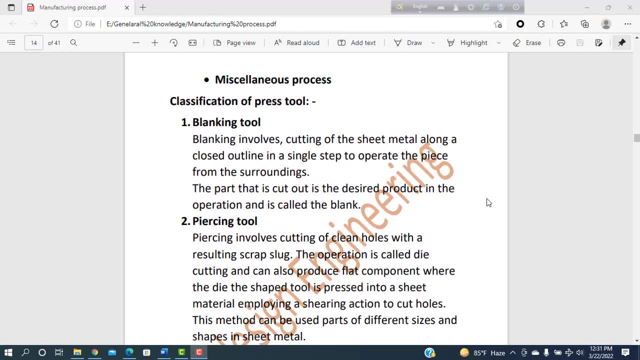 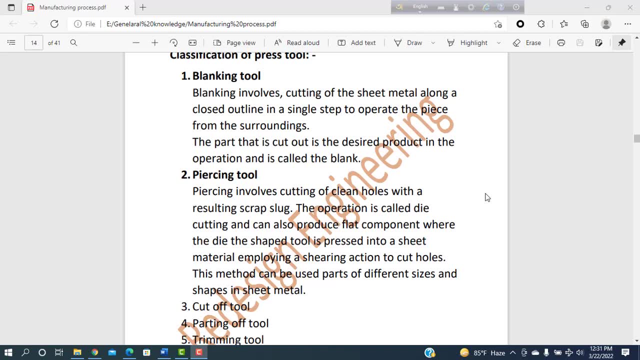 And another one is the classification of the press tool. Classification of the press tool includes that blanking. blanking involves cutting of the sheet metal along a closed outline in a single step to operate the piece from the saronics. The part that is cut out is the desired product. 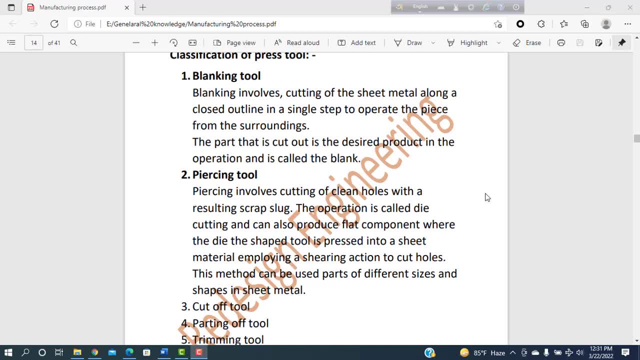